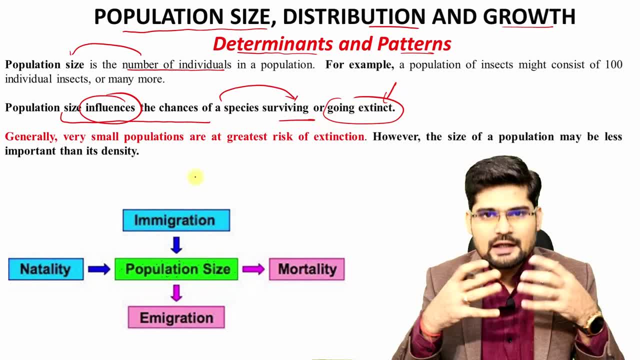 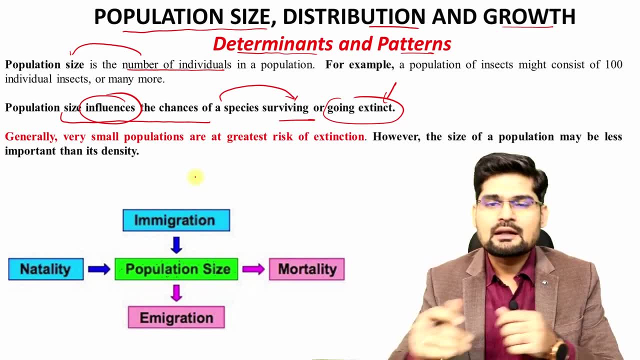 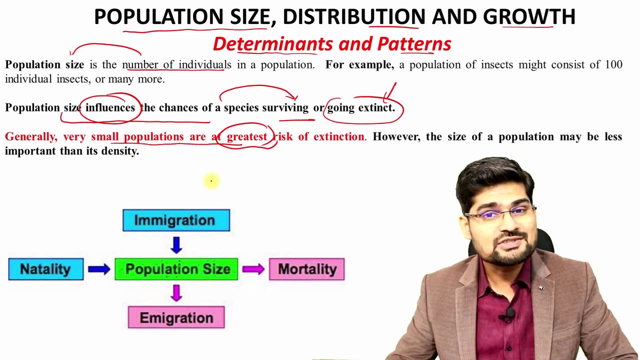 extinction. it means more people, it means we are able to survive for longer period of time. that's one probability or one hypothesis that is always given with population size. now, what is important here? to consider that very small populations are at greater risk, mostly of extinction. so, as you know that already. 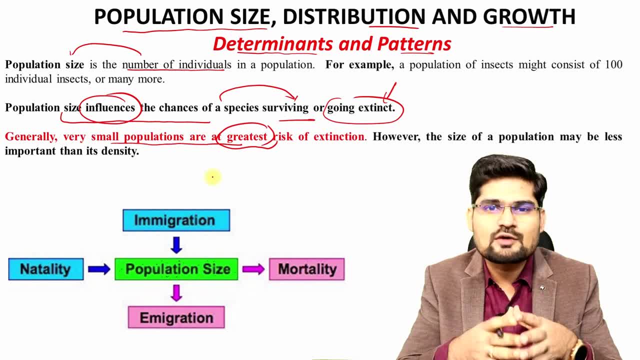 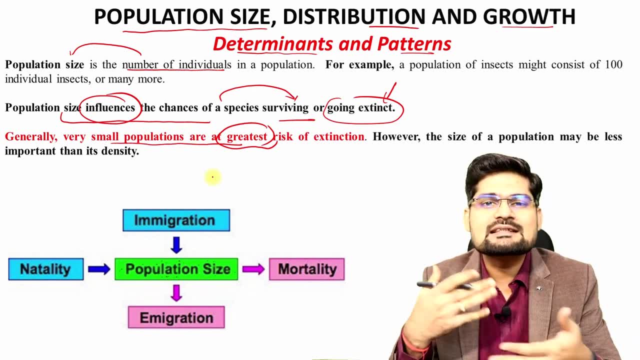 five mass extinctions have happened and if you have not watched the video on geological time scale, it's there in the geomorphology playlist. you can go there and watch it for yourself. now we are saying that this is the sixth mass extinction. now, where the population is endangered? now, gradually, population is. 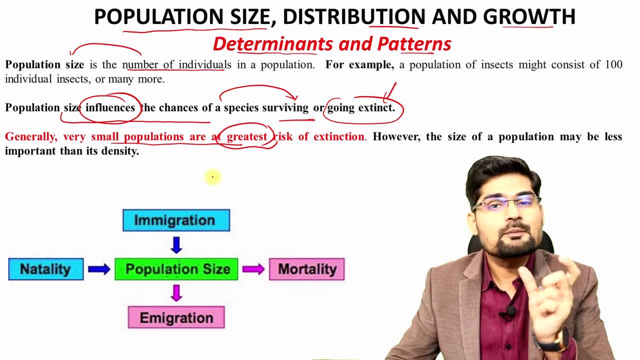 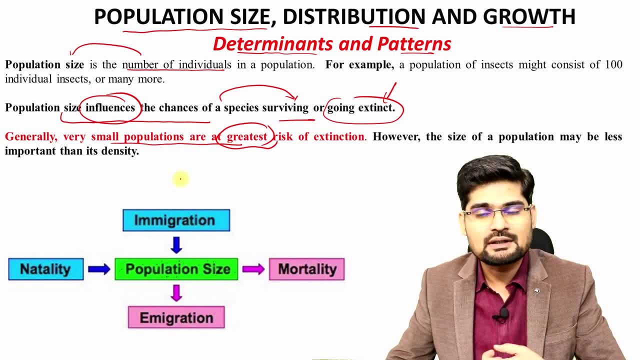 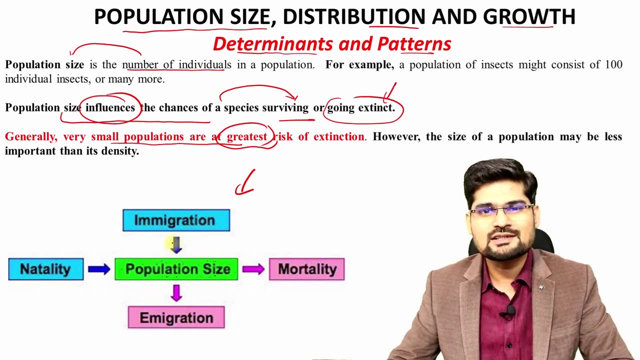 going to get extinct with time. so for population geography specifically, if we talk in human geography, human population is very important. size of population is equally important and also this is the flow diagram that we can understand in terms of the population size and the dynamics associated with its factors. 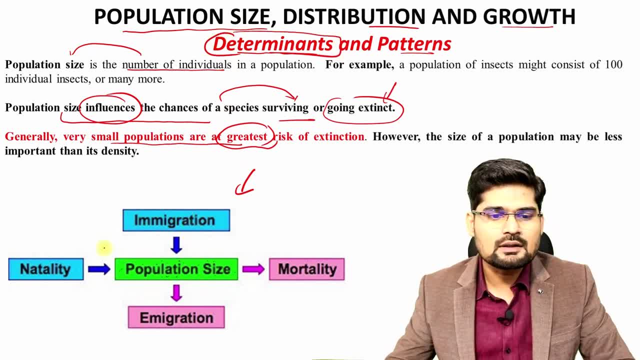 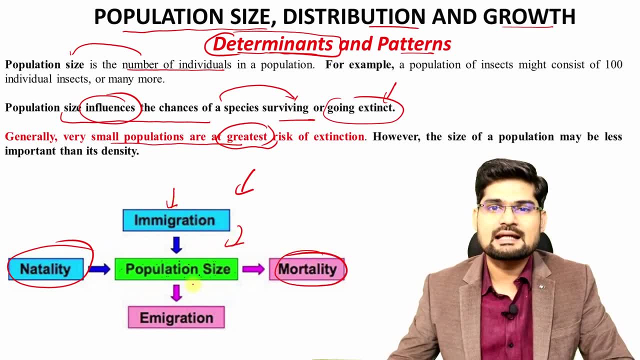 that's where we say the determinants now remember natality, that is related to birth rate, then mortality, related to death rate, then immigration- people coming inside and immigration people exiting that particular area- the balance of these particular factors, these determinants talk about that- what the population size would be of a particular state, a district, a country, a location? 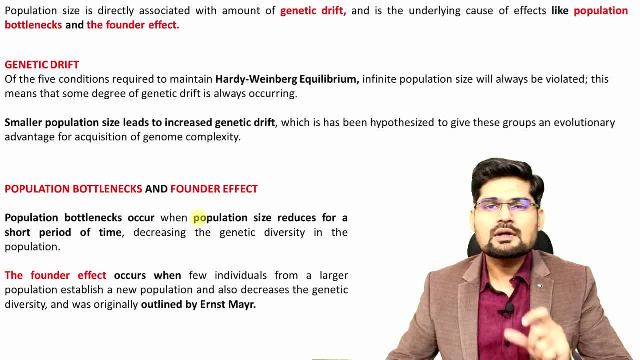 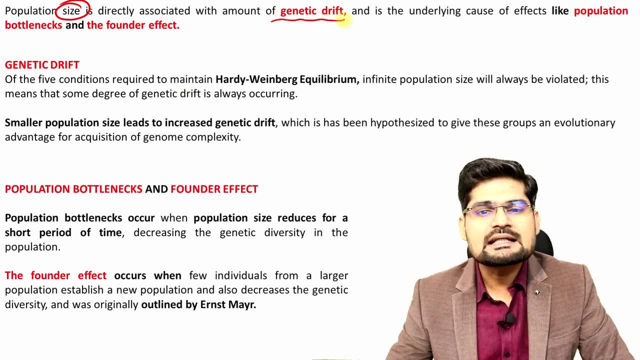 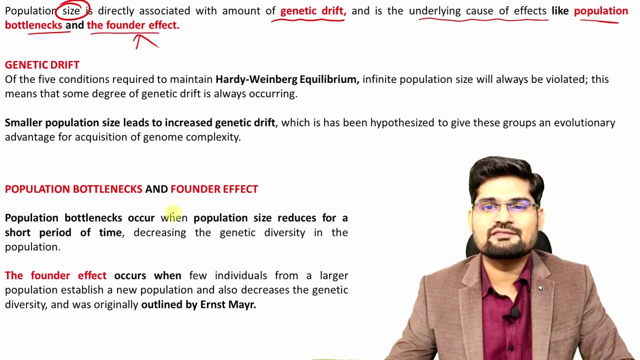 that's how we are looking into the topic now. more important points to be understood here is that population size is also directly related to a phenomenon called genetic drift, and also the underlying cause of effects like population bottlenecks or the founder's effect. now, these three things are important to understand when we say: 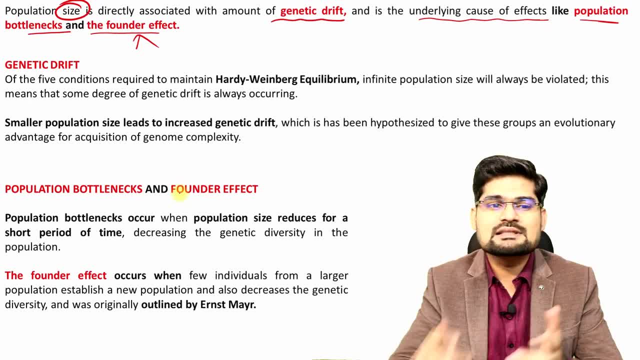 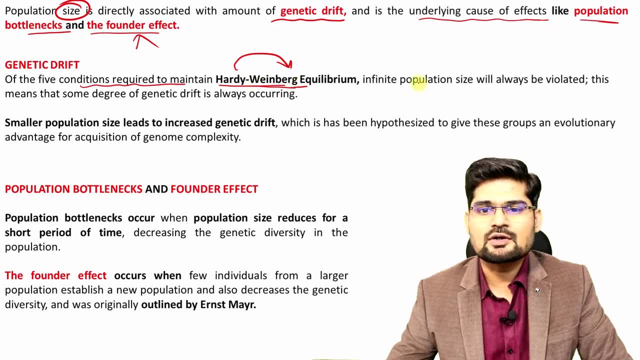 population size. what is the first thing? genetic drift. so what is it? remember of the five conditions required to maintain the equilibrium given by Hardy-Winberg? that's talking about the population size. so what is it? five conditions required to maintain the equilibrium given by Hardy-Winberg? that's talking about the 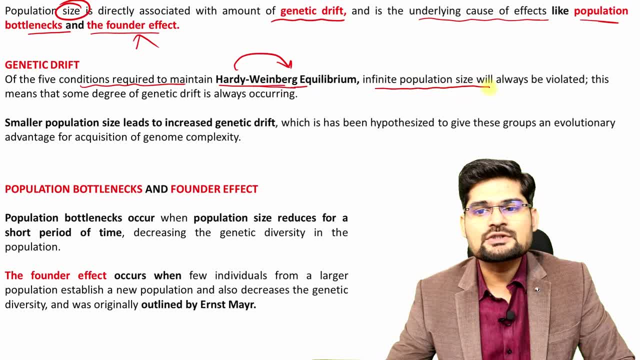 population size and its balance on the earth. So infinite population size will always be violated and this means that some degree of genetic drift is always occurring. It means what? That smaller population size leads to increased genetic drift and which has been hypothesized to give these 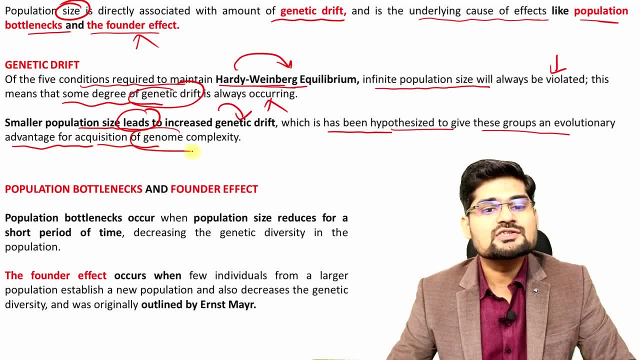 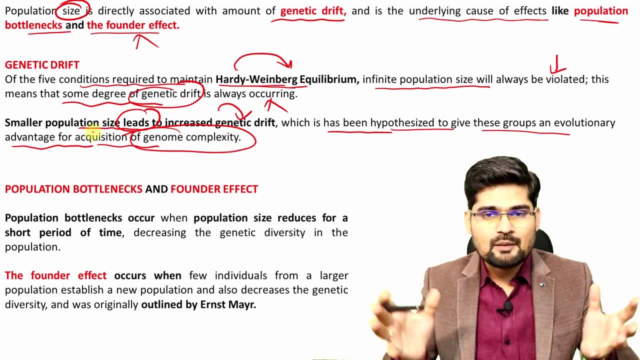 groups an evolutionary advantage for acquisition of the genome complexity. Understand that if it is a limited size, it will always have a greater chance of developing, of survival and also of the genetic drift factor. that we say right. But what about the huge size of population? 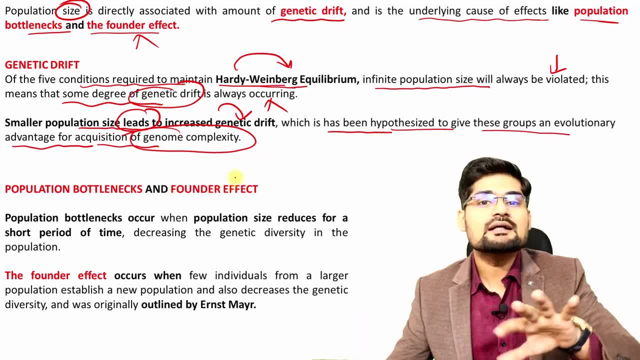 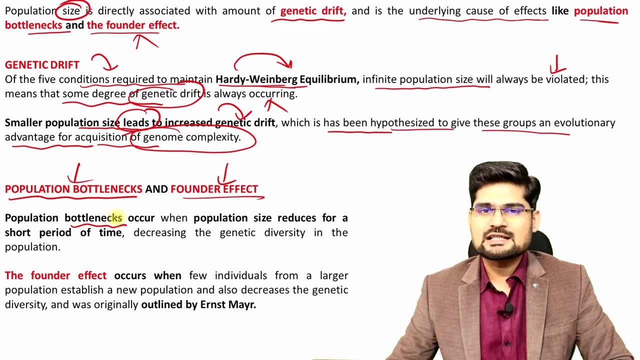 extra size, extra large population? if we have, then there will be a disbalance. Now let's talk about the other two things, that is, population bottlenecks and founders effect. What is it Now? remember, bottleneck, as we say, occurs when population size reduces for a short period of. 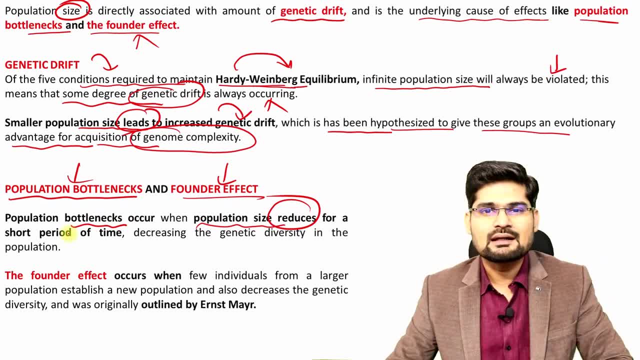 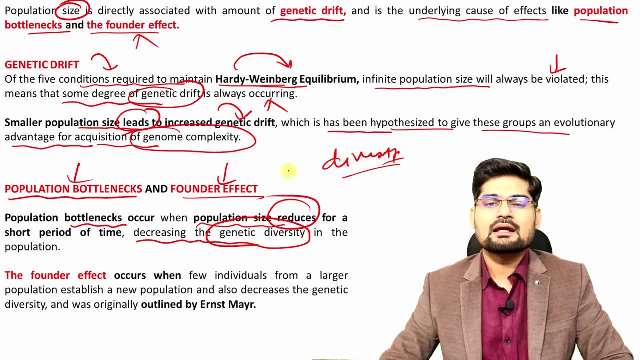 time, In a given limited time, if the population size is dipping, that is called a bottleneck right, So decreasing the genetic diversity. Now, diversity, what we understand is very important. Why? Because it gives us better chance of survival. 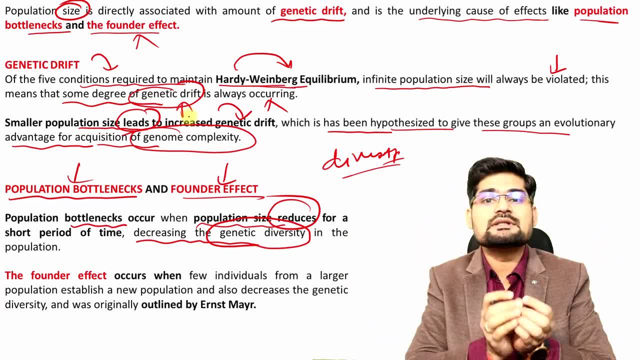 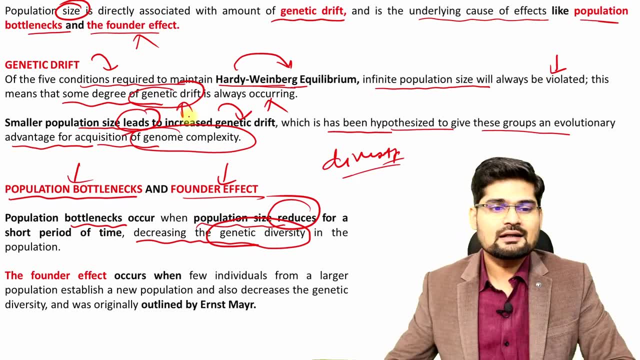 But when we say diversity, it means the as much as possible the diverse gene or gene pools, right? We have also talked in biogeography about the different gene pool centers across the planet, right? So the founders effect is what It occurs when few individuals from a large population 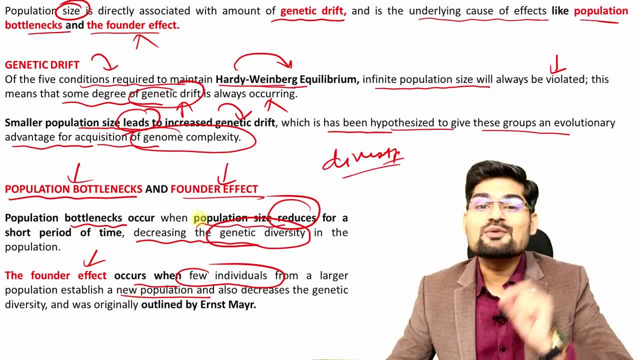 establish new population. That is called founders effect, The founder- they are the founders of the new population, They are the founders of the new population, They are the founders of the new population- And also decreases the genetic diversity, and it was outlined by Ernst Mayr. Now these are the concepts: 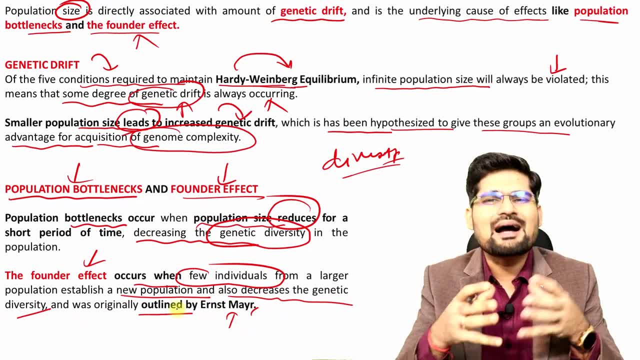 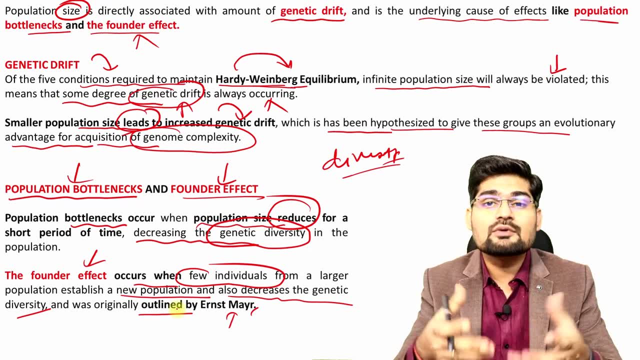 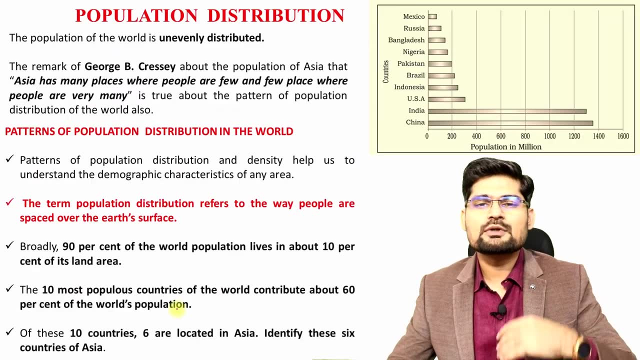 related to size of population, But sometimes we talk about it in biology, not in geography. But in geography population size is what matters for the development, for the progress of human beings and for the other associated phenomena on the earth's surface right. So when we say population, 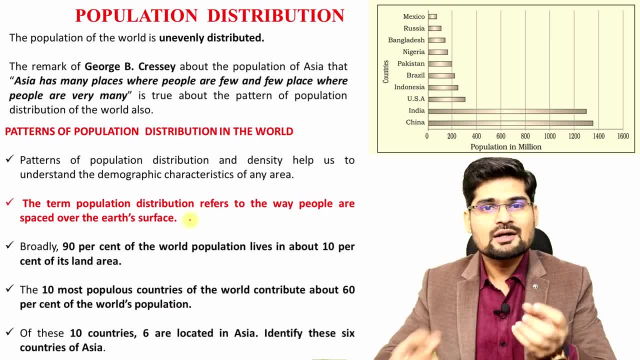 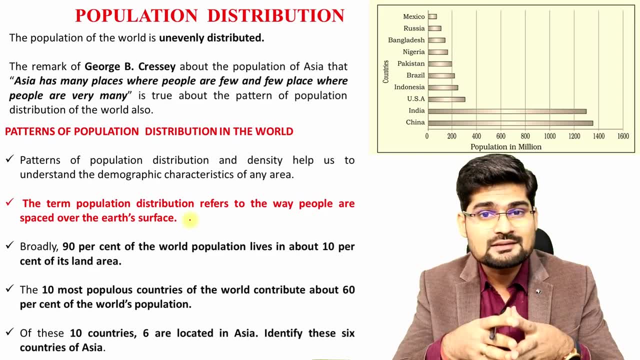 distribution after population size. what does it mean? It means that what is the location of this population size across the planet? And what is the location of this population size across the planet? Is it even? Is it uneven? Does it have some pattern which is spatial in nature, right? So population? 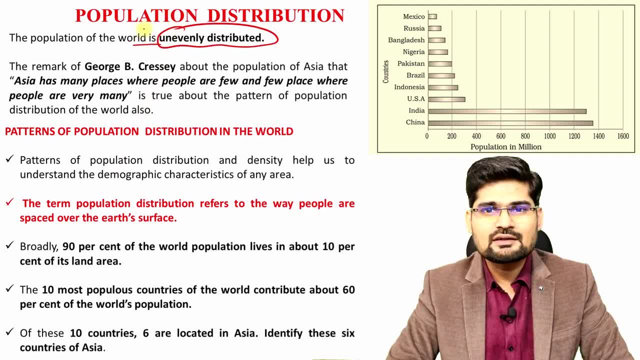 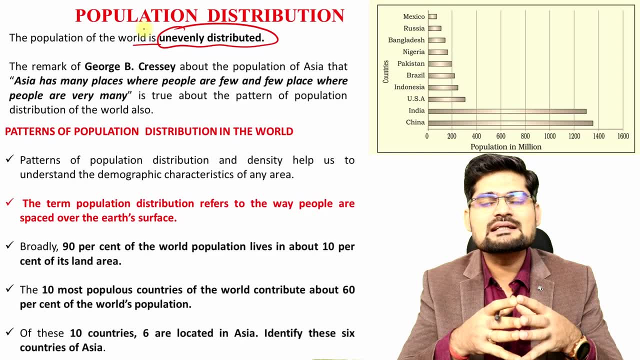 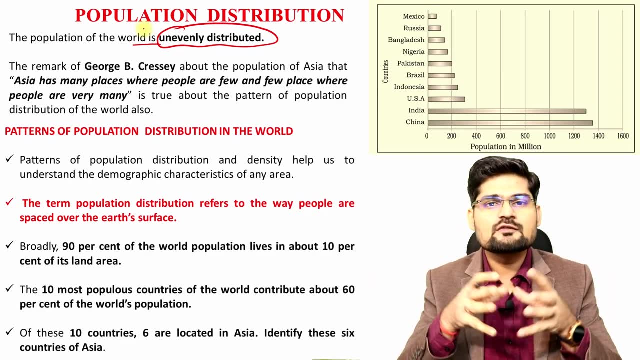 of the world is uneven, as we know. Why is it uneven? First factor that you will see is the natural factor itself: the distribution of land and water. So human beings are surviving on land. They are not the water beings. So it means what? If the land area is less, obviously people will be. 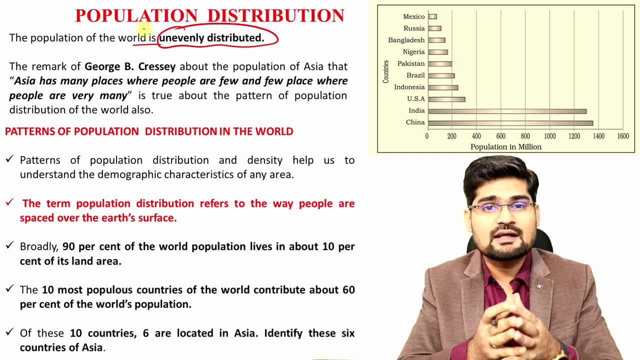 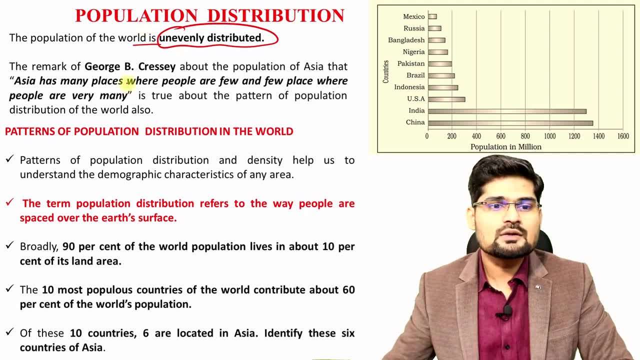 settled on land. That's the first part. Then also not all kinds of land, The specific land where the survival rate is more, it means the opportunities of survival is more. That's the natural reason. So the remark of B Chrissy, if you observe carefully the population of Asia, So Asia has. 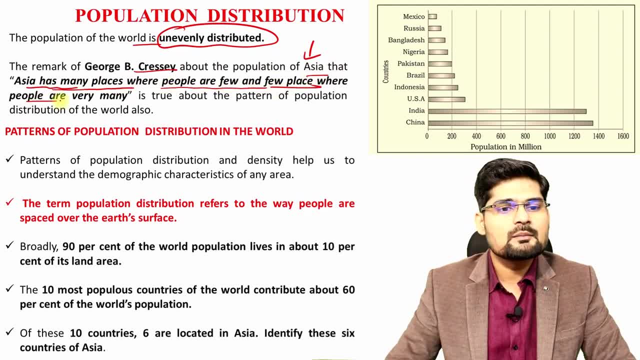 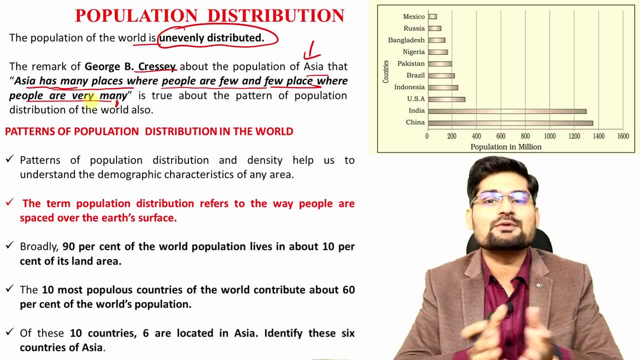 many places where people are few, few places where people are very many. Now, this is very interesting, that there are few places where people are there, and those few places are the densely populated areas, right, So that what we see here is the patterns of population distribution across the. 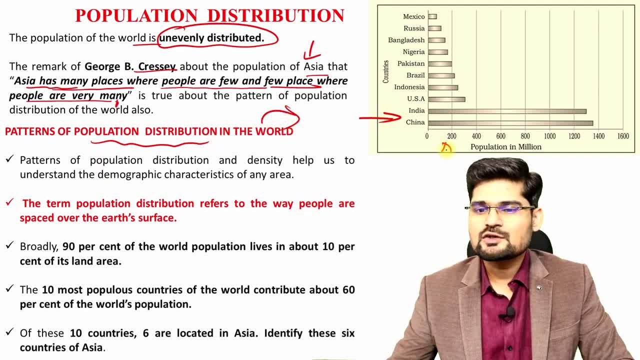 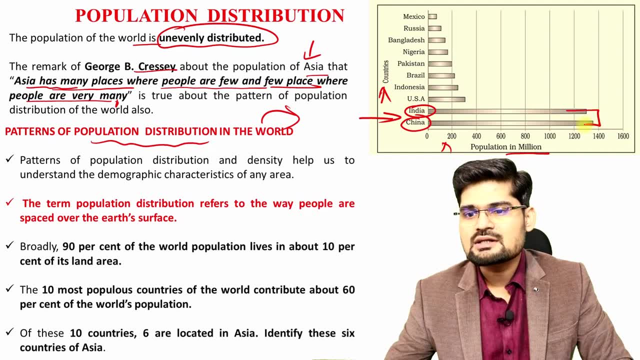 world. If you observe this particular diagram here, what do you observe? This is the population in million and this is the countries Now observe China, India, majorly two Asian countries leading the chart. So what you observe? that, apart from this, you have Pakistan. 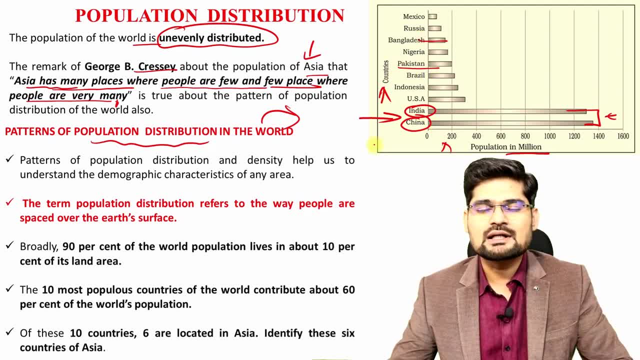 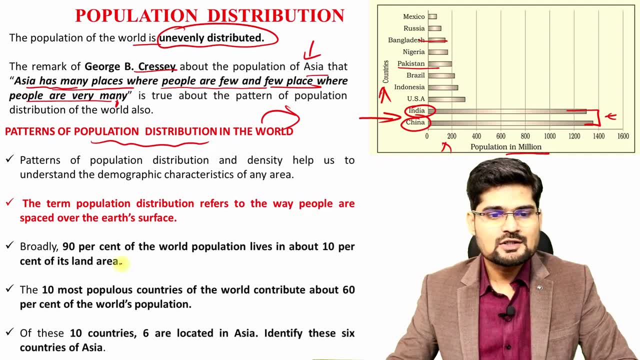 as well, Bangladesh as well. So in top 10 maximum countries, almost six countries or five countries most populated, densely populated, are there in Asia itself, right, So that's what we see: that patterns of population distribution and density help us to understand the demographic characteristics. 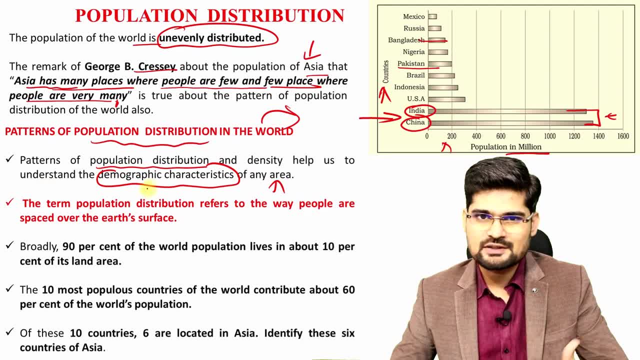 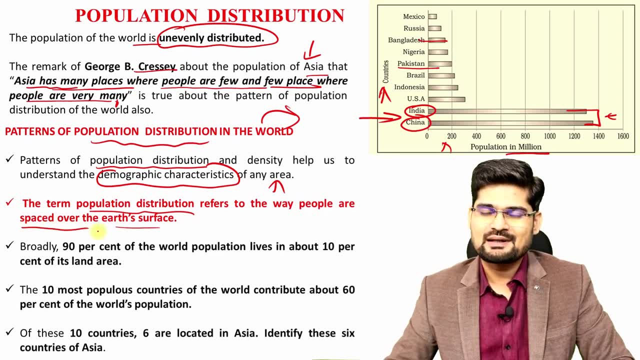 of a particular area Right Of a particular region of a particular country. So the term population distributions basically refers to the way people are settled over the space right. So we say population and settlement together many times So broadly: 90% of the world population lives in 10% of 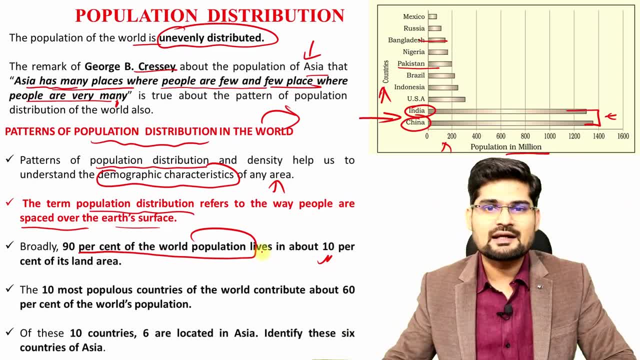 its land area. So 90% is living in 10% of land area. It means now the density of population in that 10% would be amazingly great, right? So 10 most populous countries of the world contribute. So if you look at this map of the population density of Asia, there is about 10 countries. 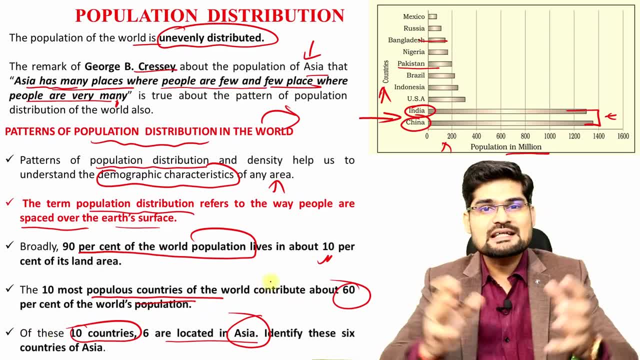 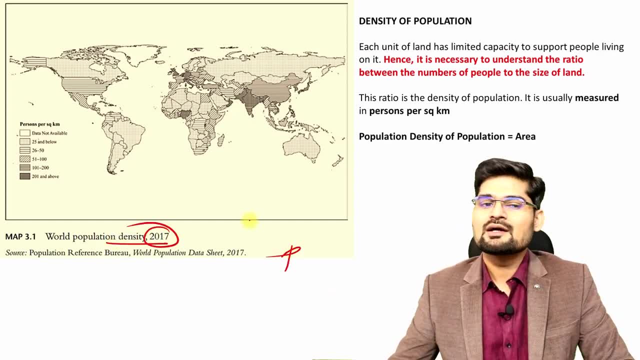 of the world and of these 10 countries, six are located in Asia itself. That's what we see: that Asia has the most population distribution across the world. So if you observe this map of the world population density 2017, what does it show? Look at this particular. 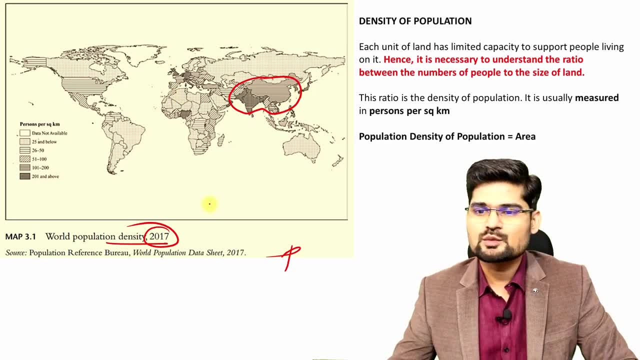 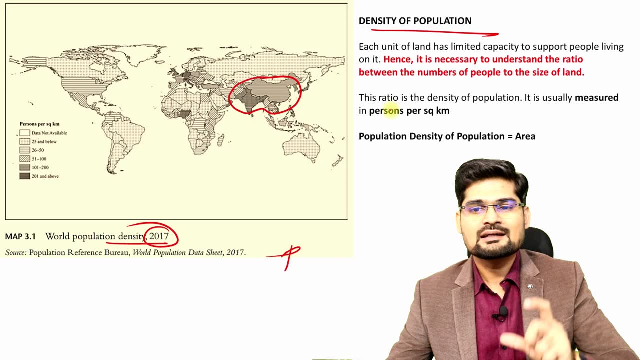 region, Asian region. It's one of the most densely populated areas of the world. right And density of population is measured in order to understand the ratio of land and human beings. right, So we also, in crude terms we say, man-land ratio. So what? we observe, the density of 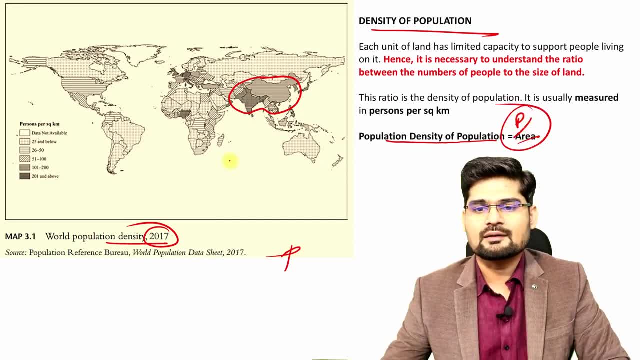 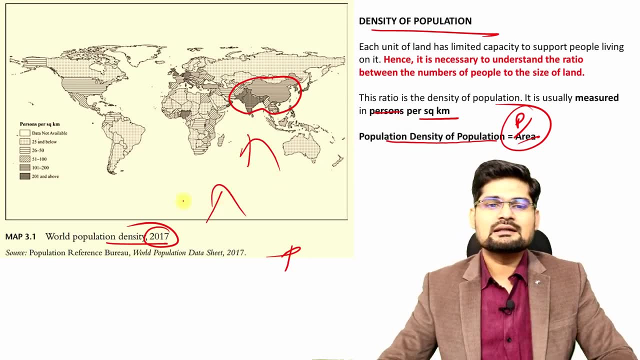 population is basically population upon the area right. So persons per square kilometer of area is what we look here. So if you observe these kind of maps, you'll find out that there are few pockets in the world which are densely populated, while rest of the world is not that. 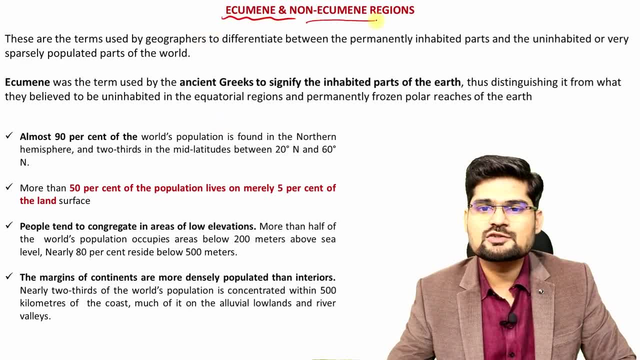 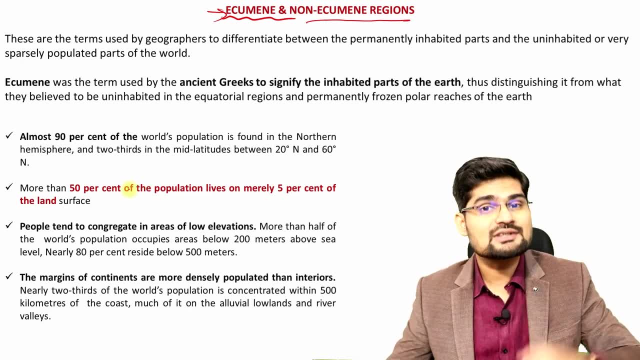 dense. And before we go into the factors of the population distribution, there are two more concepts to understand in terms of the settlements of people, The population patterns across the world, famous since ancient Greeks Remember this Yukhman region and non-Yukhman region. 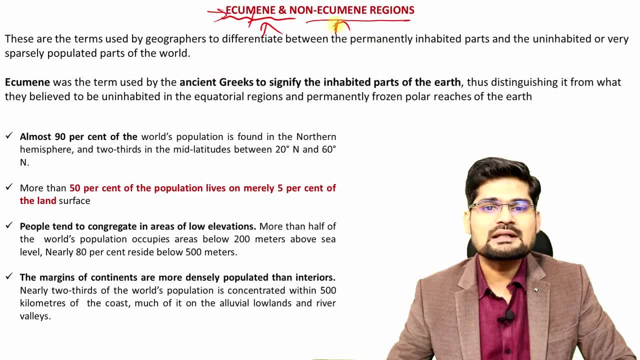 is it? It's talking about the areas of permanent settlement and non-permanent settlements, The inhabited world and non-inhabited world, which was specified by ancient Greeks right? We have learned this in the evolution of geographical thought lectures, which is also there as a playlist on my 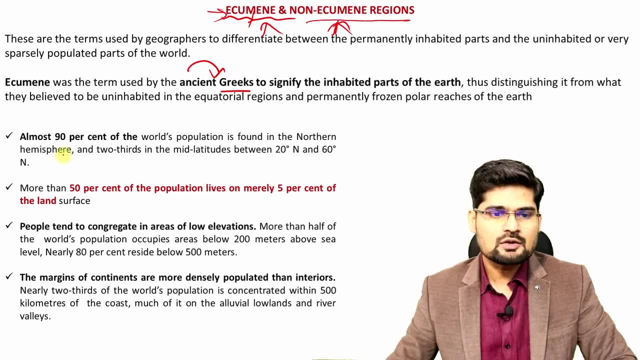 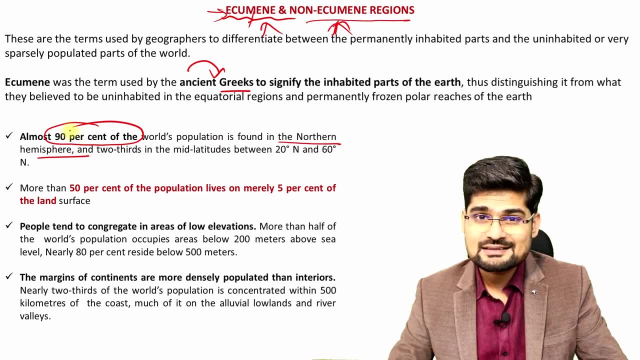 channel. If you have not seen the lectures, you can go there and watch it as well. So almost 90% of the world population is found in the northern hemisphere, where you have more land areas, right, So two-thirds in the middle latitude between 20 to 60 degree north. that's very important. 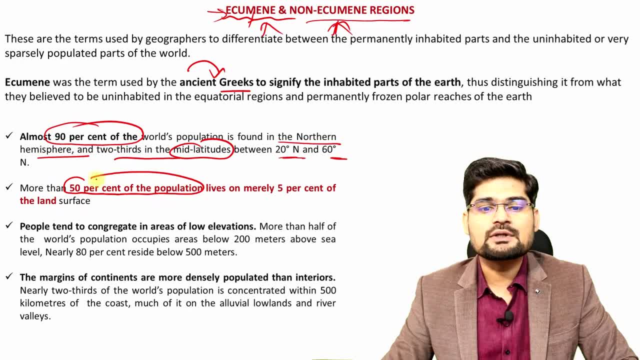 geographical location and 50% of population or more lives merely in the 5% of the land, So understand it's concentrated in particular belts right, and people tend to congregate in areas of low elevations as well as margins. of continents are more densely populated than the. 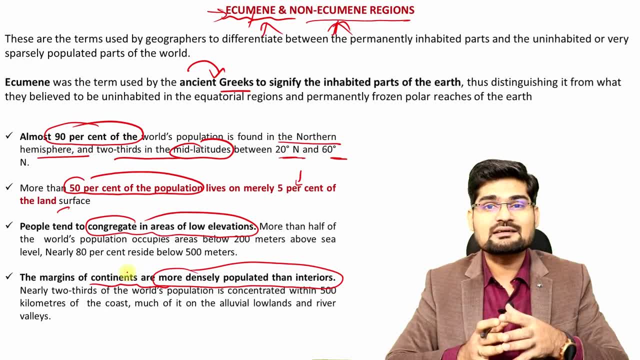 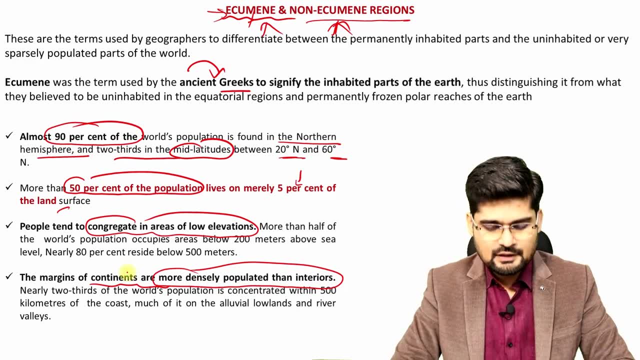 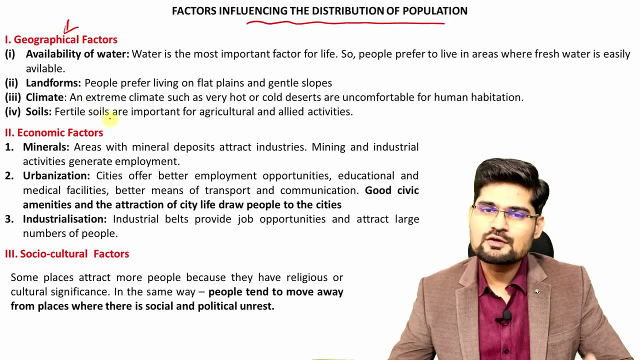 interiors, So continentality factor, and coastal factors, So margins are more densely populated than many interior areas, Areas of the world. that's a general pattern, if you observe. So now let's look into these factors influencing distribution of population. So first is the geographical factors, and of course we 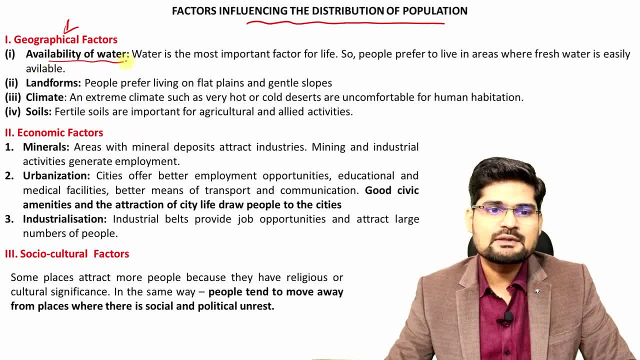 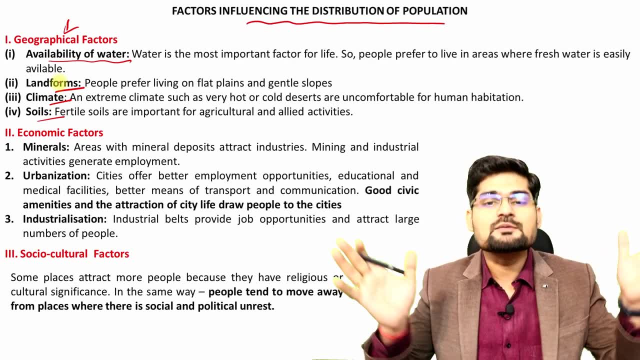 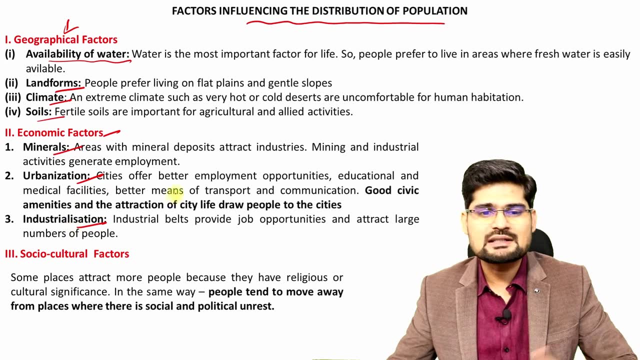 understand geographical factors, like physiographic factors such as availability of water, landforms, climate, soil. So if these are conducive for human settlement, obviously it will host more people, right Then economic factors like minerals, urbanization, industrialization, job opportunities. 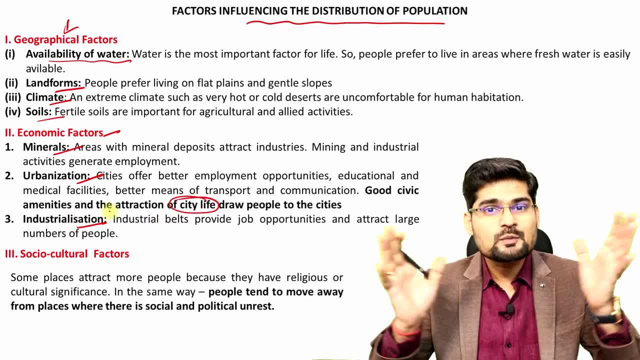 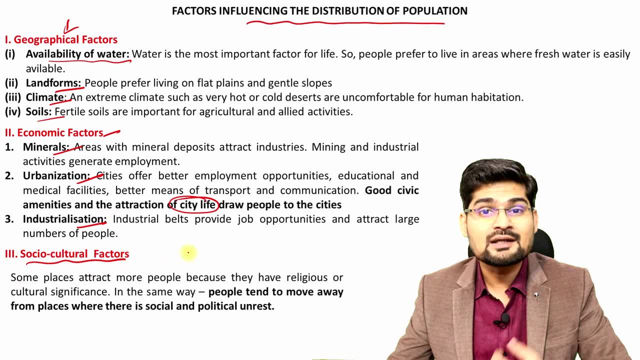 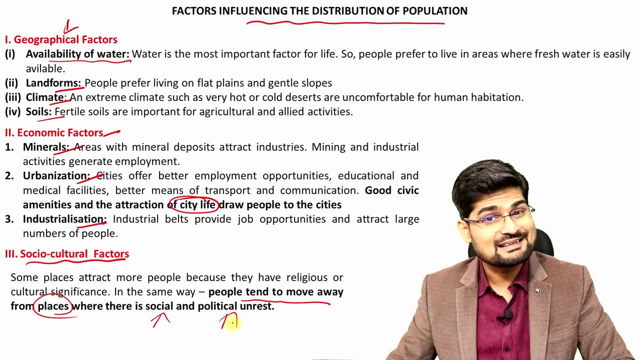 amenities, attraction to city life. This is where more people are being concentrated in urban areas. right and sociocultural factors, For example, social harmony, cohesion between people, and remember people tend to move away from places where there is no social harmony. and if there is unrest, right, So peace is also. 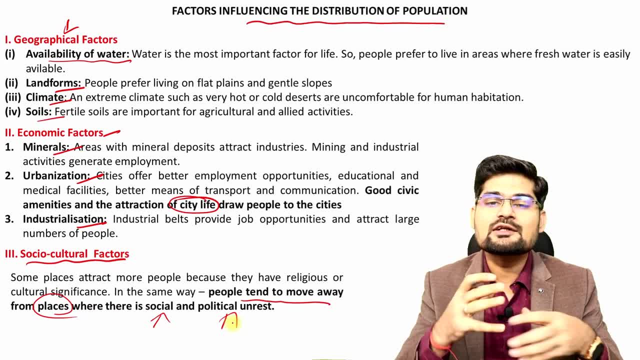 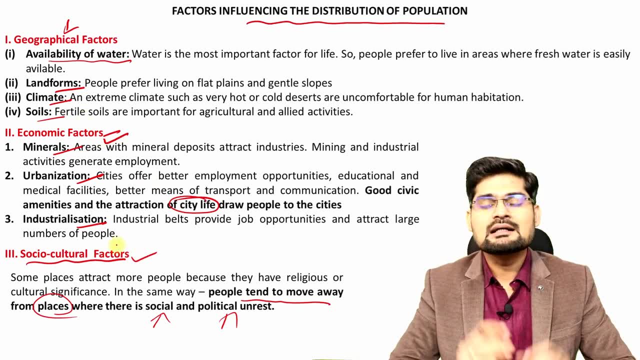 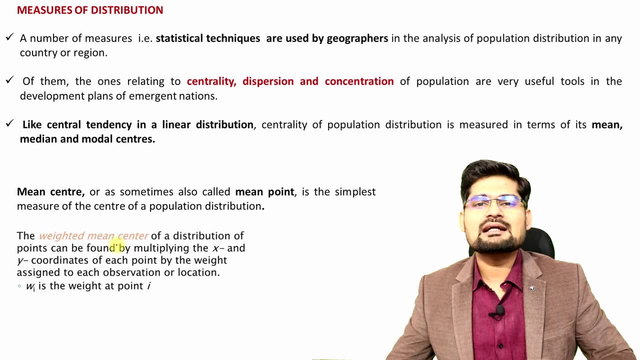 important for people's settlement right. People would not like to reside in an area of conflicts, So that's what the geographical factors, economic factors and sociocultural factors are The determinants of these: population size as well as density, as well as distribution. right Now, let's understand some of the measures. 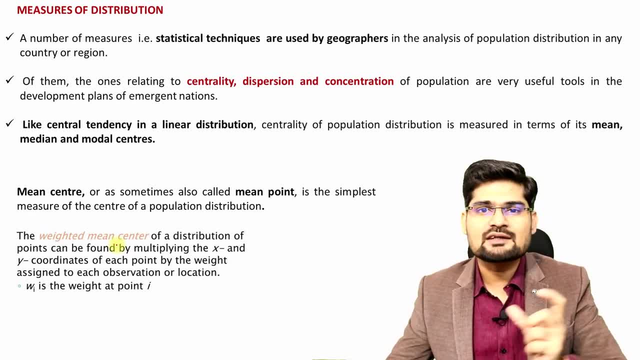 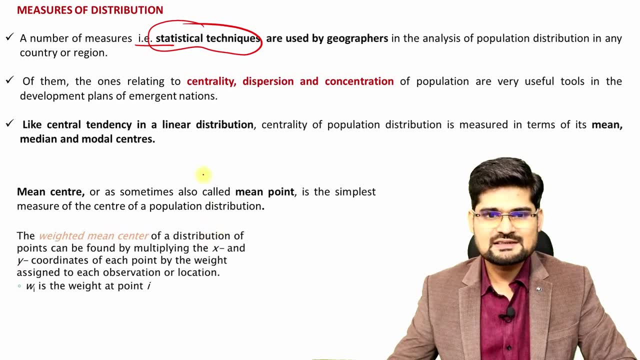 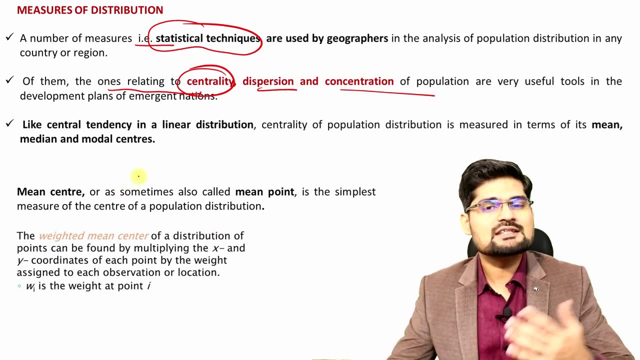 that we take in geography to understand or measure these kind of distribution across the globe. So number of measures are there, especially based on statistical techniques used by geographers. So, for example, we have measures of central tendency, measures of dispersion, the dispersion and concentration of population as very useful tools. So measures of central tendency, basically. 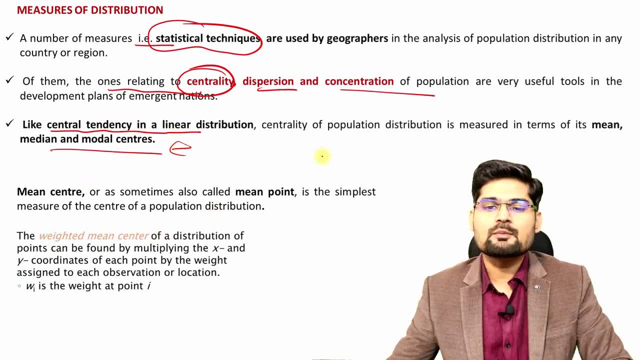 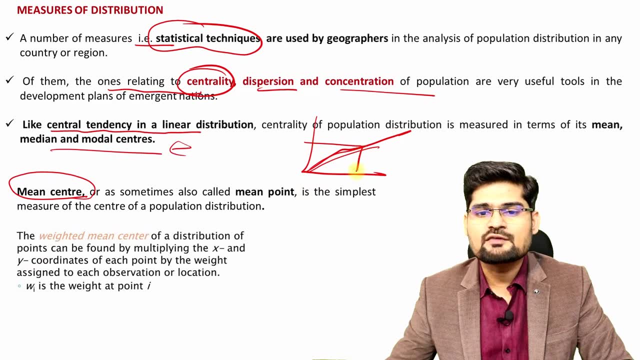 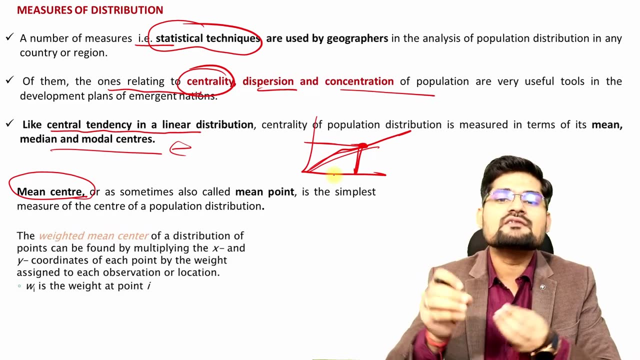 we talk about the mean median mode, Right? if the population is centered around a particular distribution or not, right? So mean center also is sometime used for mapping technique, right? If we want to plot a mean center, it will give us an impression that if the population of that particular area is centered around mean, 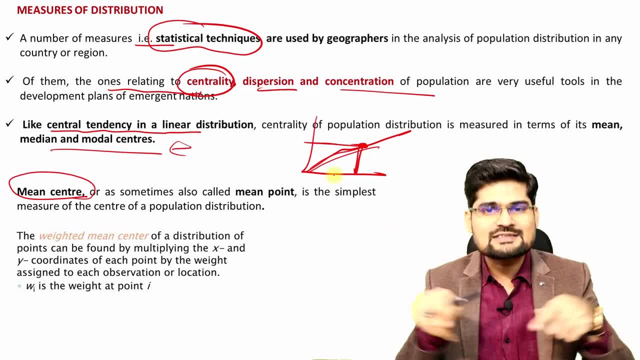 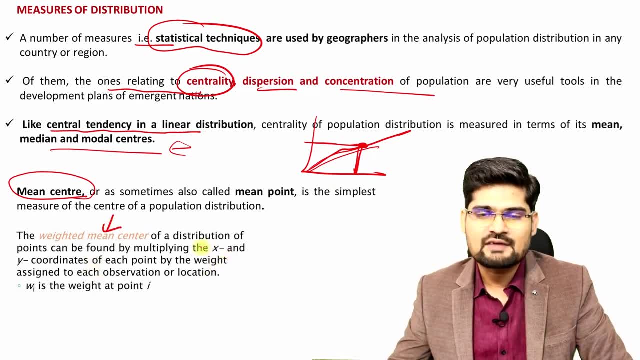 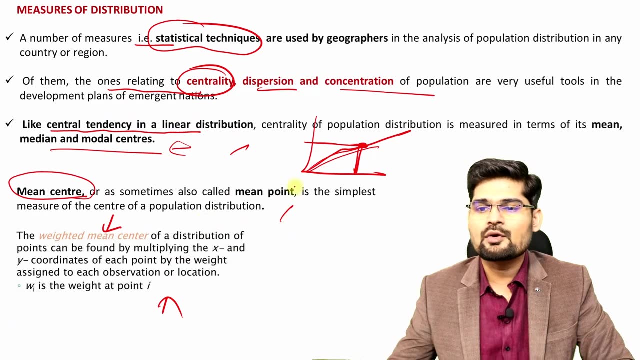 which area is the mean center of a given state or a district which we can plot through this mean center, or median center as well, or weighted mean center, alongside some of the important factor of multiplication is used right So that also we can utilize In details if you want to look into the mean center and mean point. 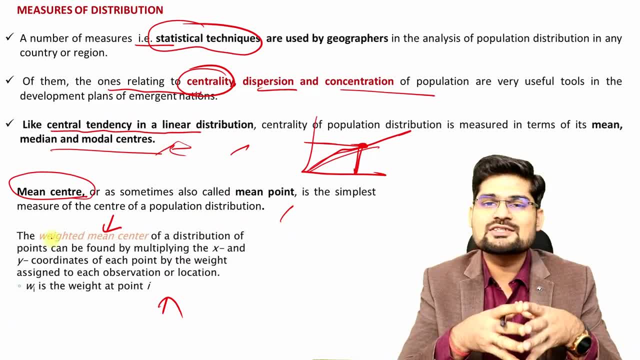 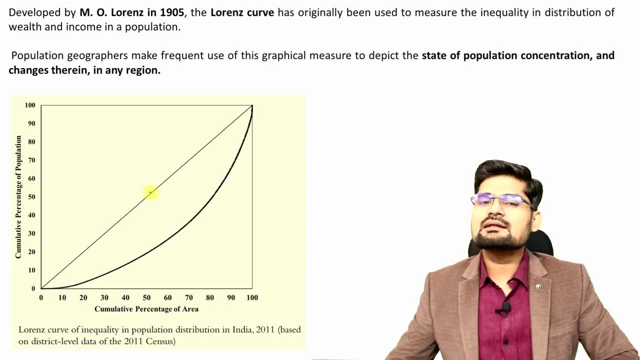 and also mean median mode. you can take any statistical techniques in geography book and there you can study it in details that how these are calculated using a population data. Now, another important thing here is the Maxo-Lorentz curve 1905 which was given. 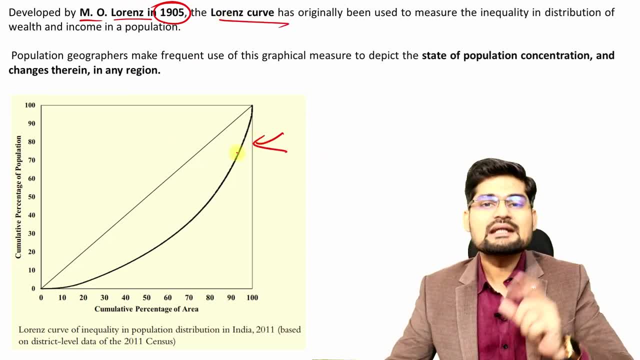 So this Lorentz curve is this curve, if you observe right. and many times this is also an indicator of how the population is equally or unequally distributed. So measure of the population is equal or unequally distributed. So measure of the population is equal or unequally distributed. 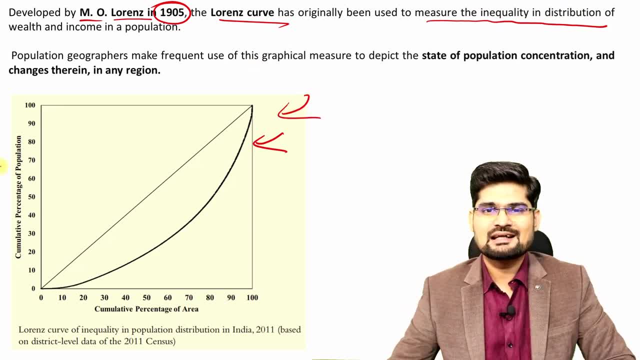 So measure of the population is equal or unequally distributed, Measuring the inequality of distribution. we many times use this right, So state of population concentration and changes in any region is also represented through the Lorentz curve. If you observe, this has been plotted for the 2011 census, that is, for India. 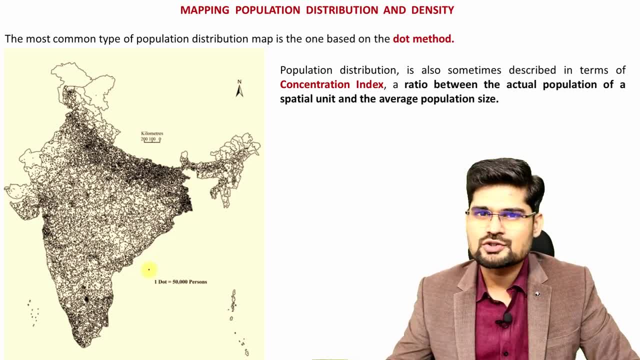 Now, mapping population density and distribution is very important in cartographic techniques as well and very famous in population geography. So the method is also called dot method. So representation of the population density is very important in cartographic techniques as well. The method is also called dot method. 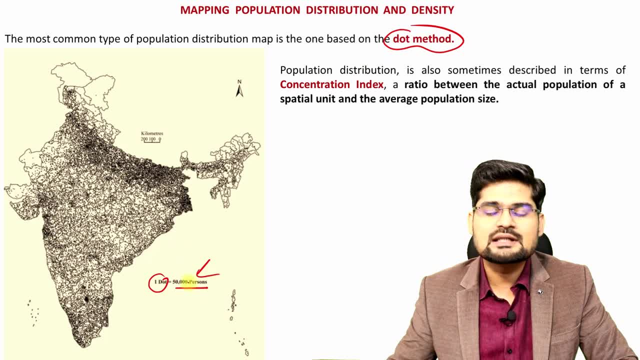 through these dots, plotting the dots in accordance with the conversion in terms of number of people, so one dot representing a certain number of people- and then making these dots in terms of where they are distributed. so this is one way where we can say that if this area is densely populated, it can be 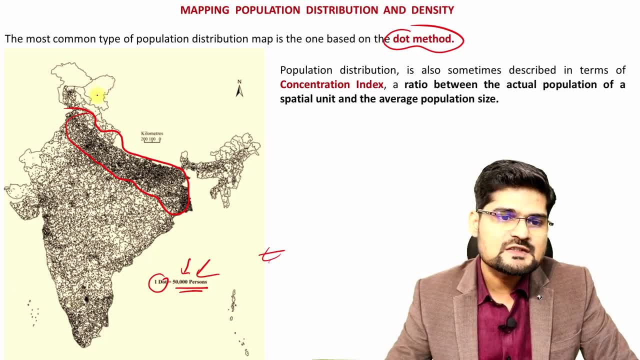 shown through the dots. for example the Ladakh region which is sparsely populated- you see very few dots. but what about northern plains? extensively there, right in central India, sparsely population again. coastal India, densely population, right. so these kind of spatial patterns can be just given by 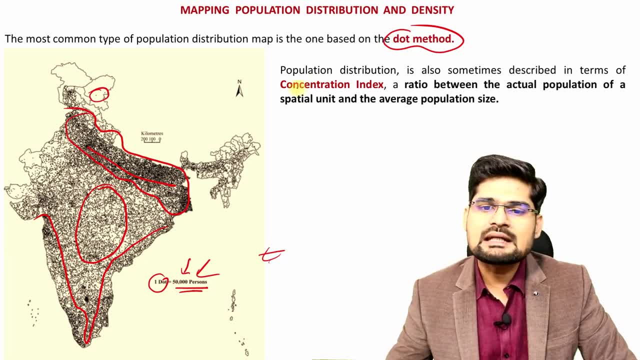 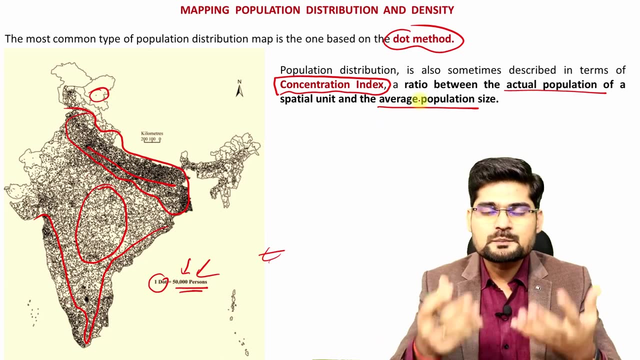 the plotting of dot method right. and also many indices are created, for example concentration index right. it's a ratio between the actual population of a given area and the average population size. so if these kind of indexes we can prepare, it gives us how to actually map it and speak for itself. that how the 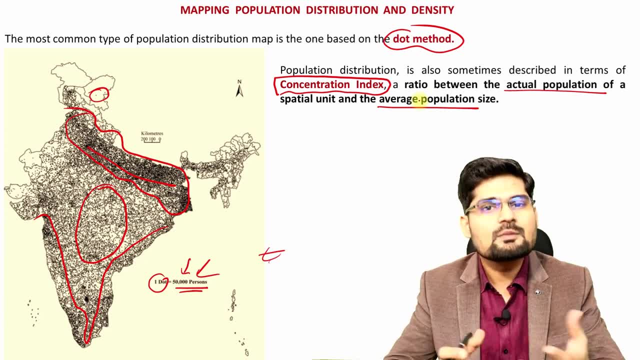 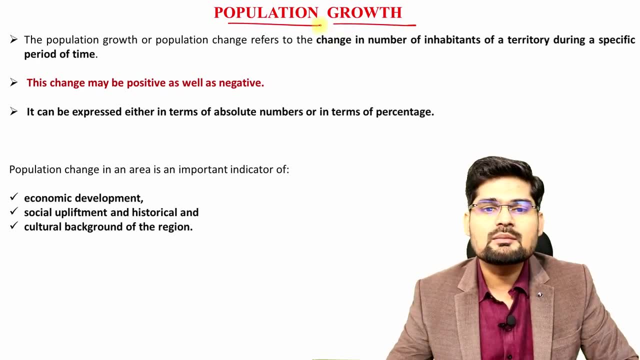 patterns look like on particular areas, area from global to local level. now what we look into. the third thing is population growth now. when we say growth now, remember it's very important to understand- we have already talked about it- what is the difference between a growth and development. so growth of population change refers to the change. 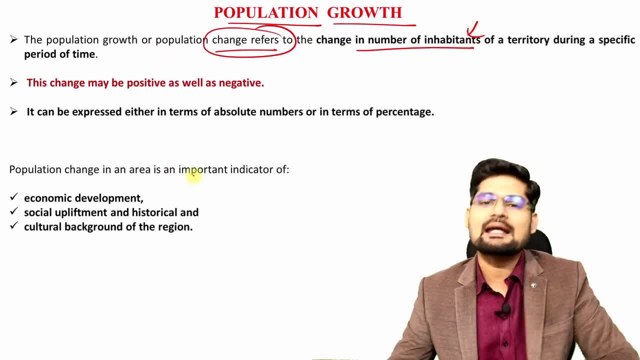 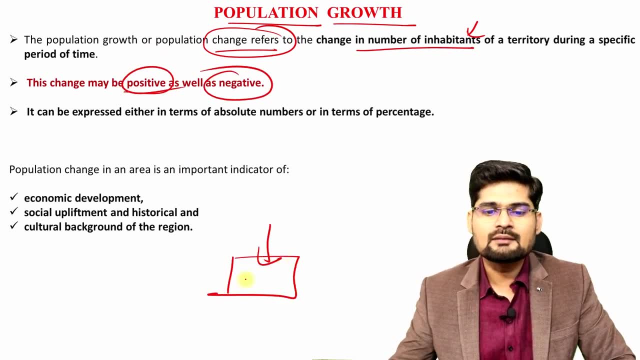 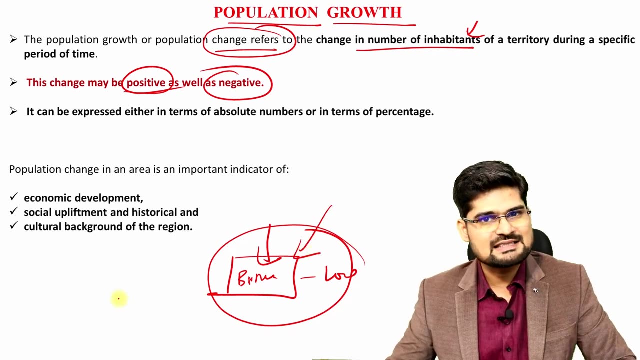 in number of inhabitants in a given territory over a specific time period, right so this change may be positive as well as negative for instant, if this is an area, if people are coming in right, and if birth rate is high and death rate is low, it means very high population chances of this area, right so? 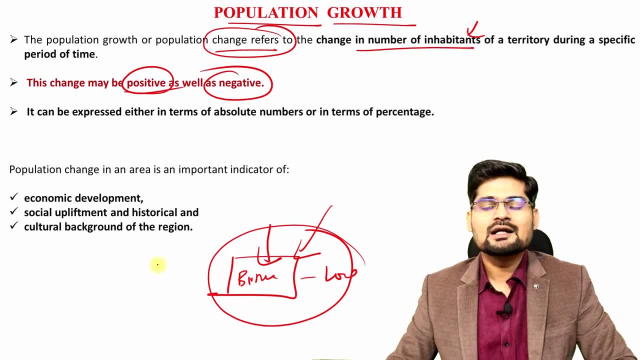 this is how we look into the change of population in an area, depending upon birth rates, death rates, immigration and immigration right. so this is how we look into it, and it's percentage is generally taken in terms of absolute numbers. many time we don't take in terms of percentage it is represented, so 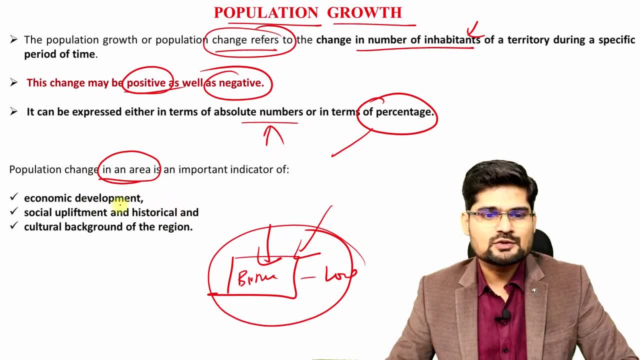 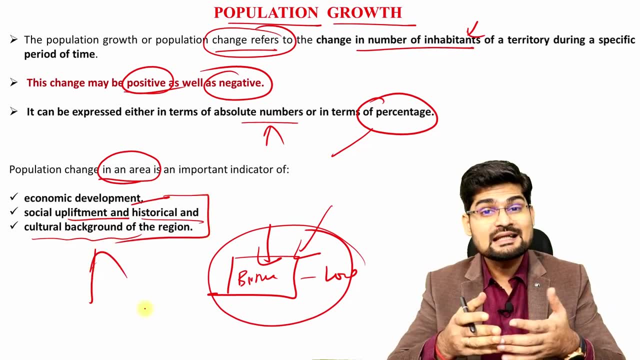 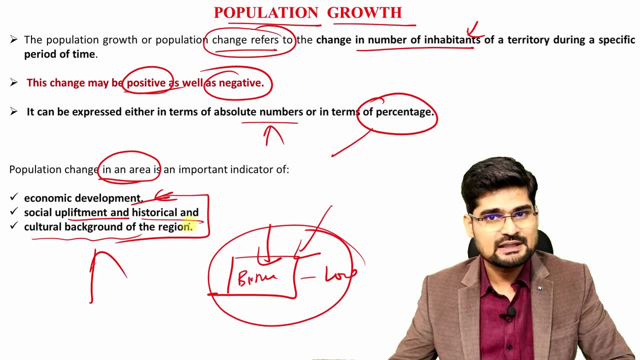 population change in an area is represented by population growth. so economic development, social upliftment and historical factors and cultural background of the are the factors, or what we say is the determinants, of population growth in an area. if an area is economically developing, obviously the population growth will be there. look at the urban centers. 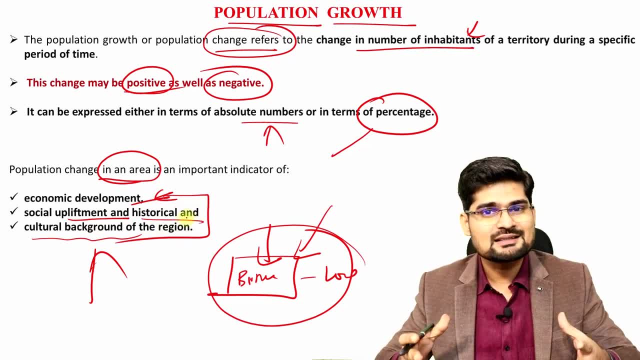 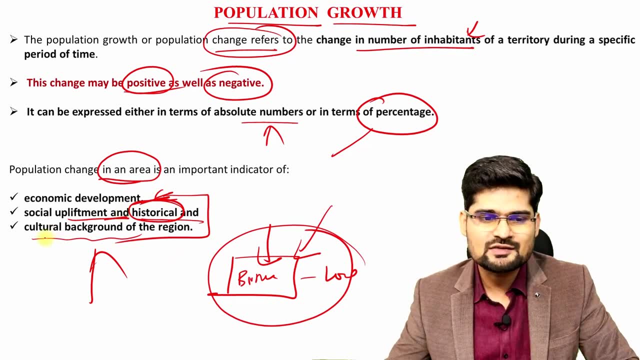 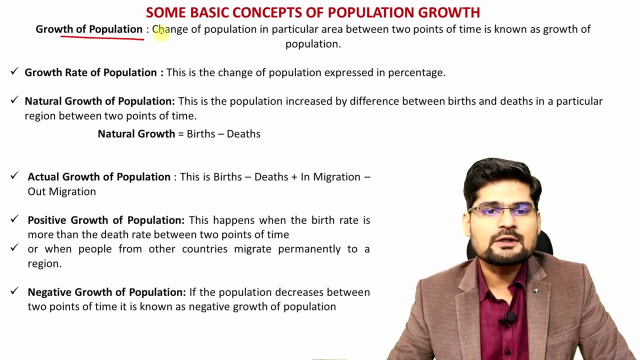 metropolitan cities where the population growth is tremendous because of so many opportunities, economic development, social upliftment, and also many places because of historical reasons you will have and cultural background of the region. so some basic concepts of population growth. if you look into the growth of population, simply the change of population in particular area, 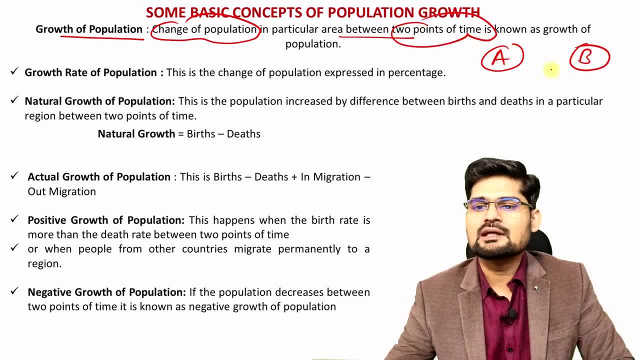 right, two points of time, so point a and point b. if you look into the base here, if say 2011 and then 21, we subtract from this population to this and we see how much is the change, so what kind of growth we can observe. right, that's how we calculate growth in simple ways. so growth rate of 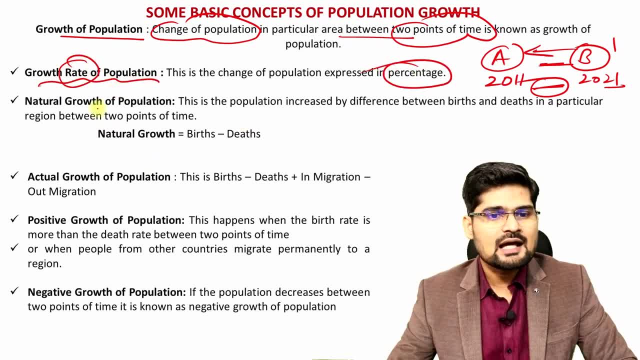 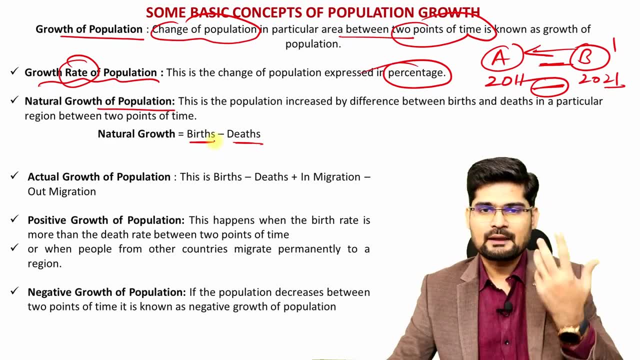 population. when we say rate, we express in percentage. natural growth of population is what basically simply birth minus death. that is what is natural. natural growth of population is what basically simply birth minus death. that is what is natural. it's not human right. what is then human? remember, when we talk about migration involved in this. 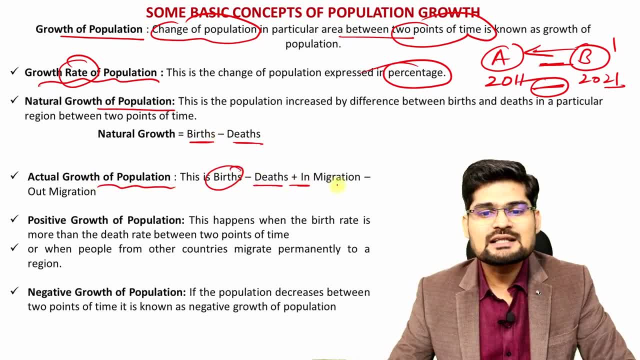 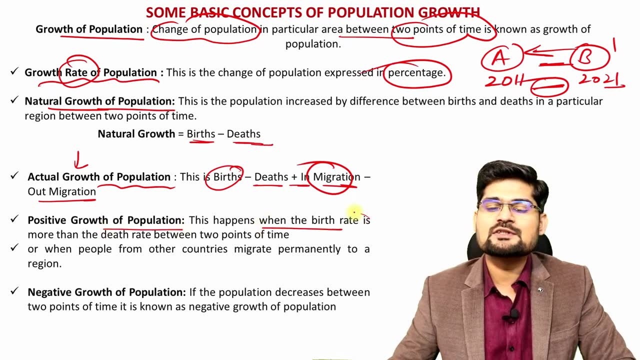 right. so actual growth of population is the birth minor death plus in migration, out, migration involved together, right? so that's where actual is there. this is natural, simply birth minus death, but actually migration factors will also be counted and positive growth of population. obviously this happens when birth rate is more than death rate between two points of time. 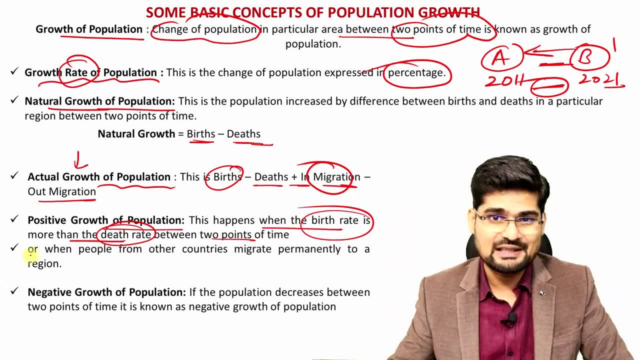 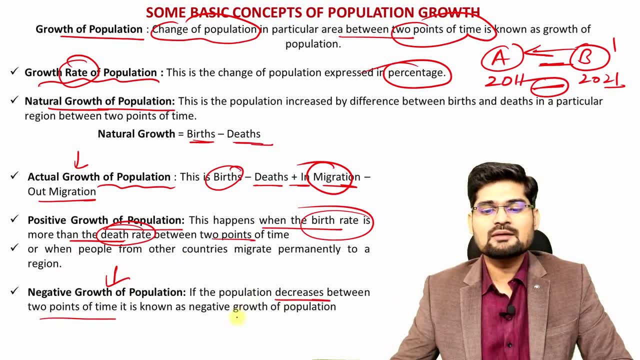 or if people are more incoming than people outgoing of the area right and similarly, just opposite is the negative growth of population. it means population is decreasing between two points of time. that's what we say is negative growth. so these are certain points or certain vocabularies that we are interested to learn in. 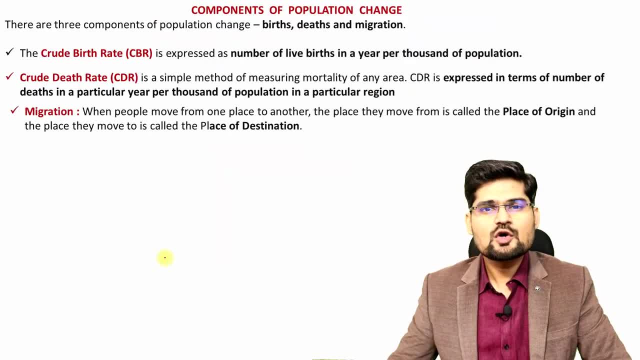 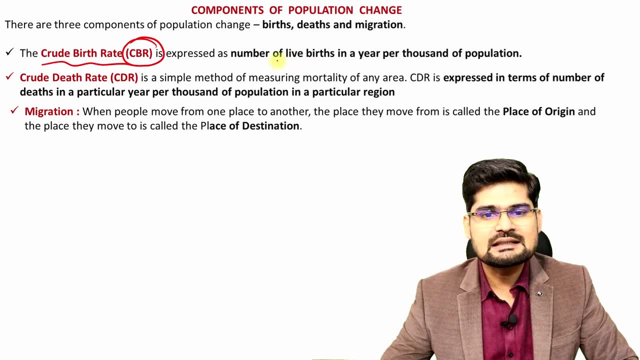 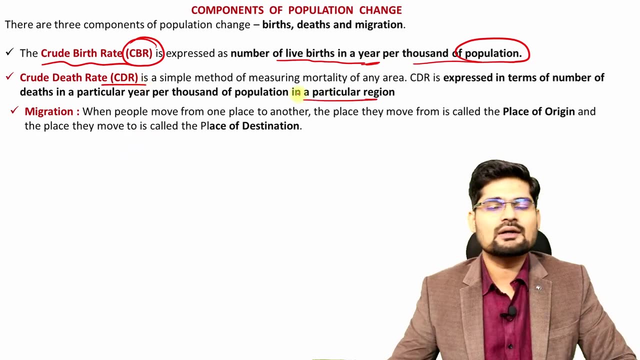 population geography related to population growth, so components of population change of population growth. if you observe, as again crude birth rate, also called cbr, which is represented in number of live births in a year per thousand population, again crude death rate in similar way is also similar ways right, according to what we observe is terms of number of deaths, in particular year. 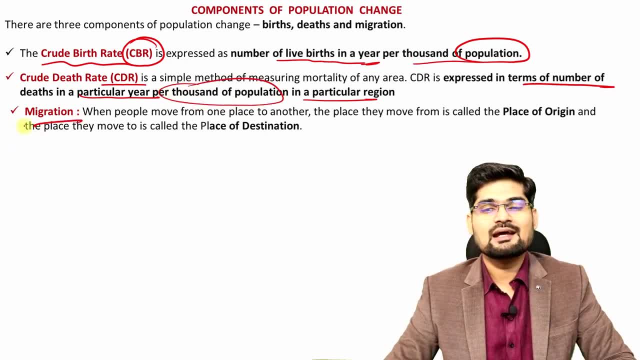 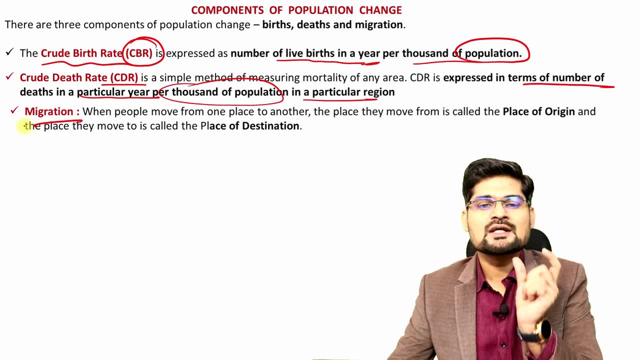 per thousand population in a region and migration right and migration in details we are going to learn in the lectures to come. also, migration theories will be learning in population geography. so migration is movement of people from this place of origin to the place of destination right. these are the factors that account for population change. population growth in an 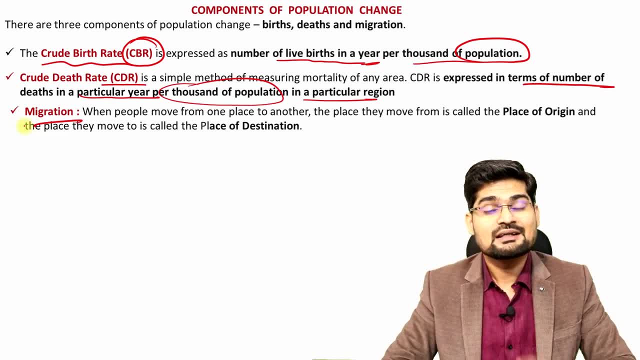 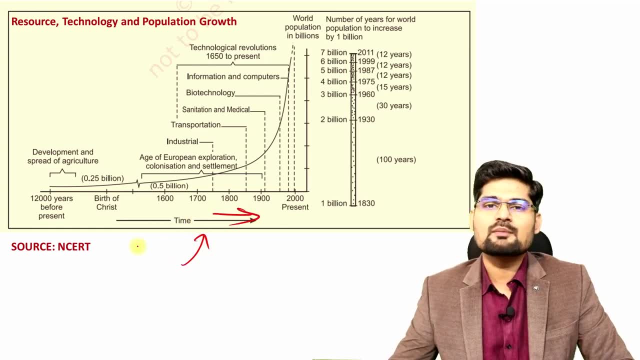 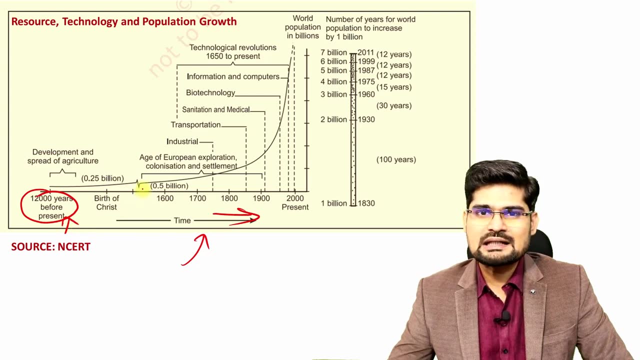 area and growth could be positive as well as negative. that's important too understand. and finally, what we look here is this particular graph. you must have seen this temporal graph of population change across the world. what does it say from the twelve thousand years when we became agrarian community, about ten thousand bc? and since then, what has happened?